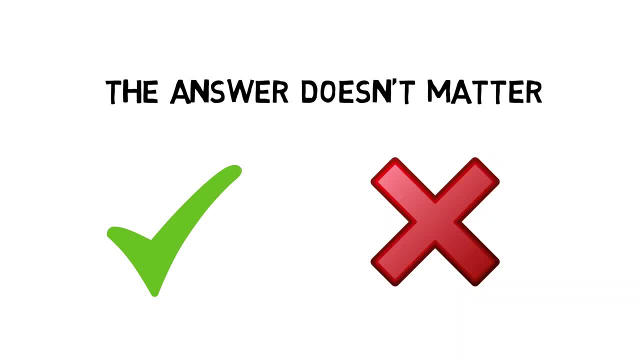 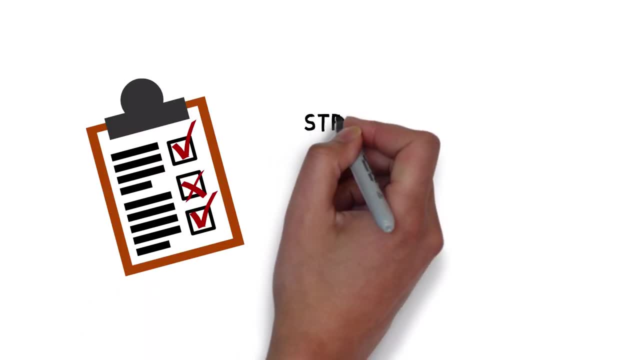 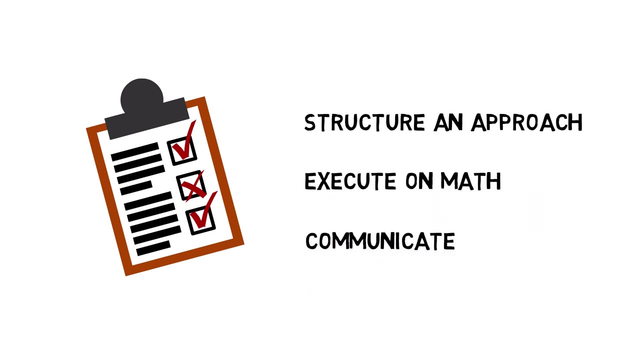 you give, Whether your answer is correct or off by orders of magnitude. interviewers use these types of questions to assess three things. Interviewers want to see you structure an approach to the problem, execute on the math correctly and clearly, communicate and walk them through your work. 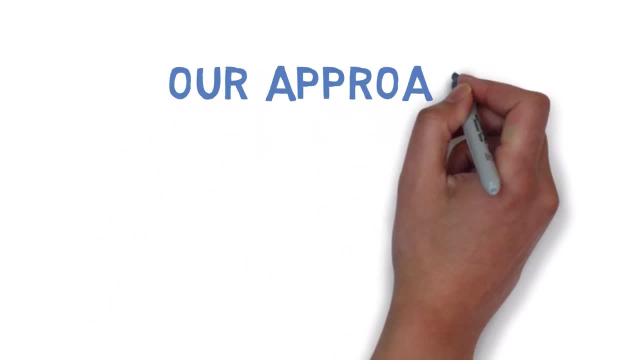 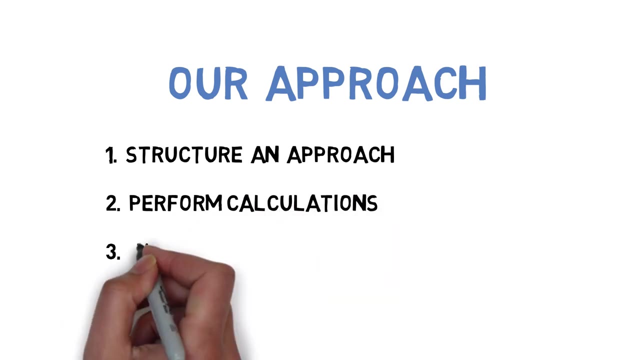 Knowing this, we can set up our strategy for tackling these pesky market sizing questions. We'll first structure an approach, then execute on calculations and, in the process, focus on walking the interviewer through our thinking and calculations. Let's use this strategy to answer a simpler market sizing question. 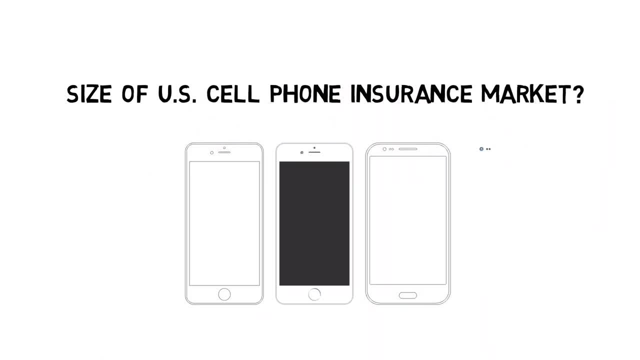 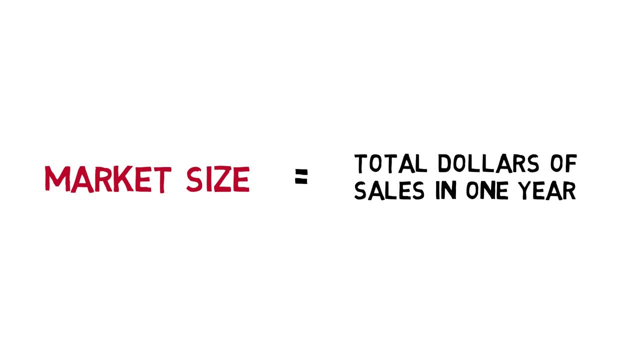 What is the market size of cell phone insurance in the US? Remember, market size is usually defined as the total dollars of sales in one year for a particular product or service. Let's start with structuring our approach first. This is the hardest part of any market sizing, or 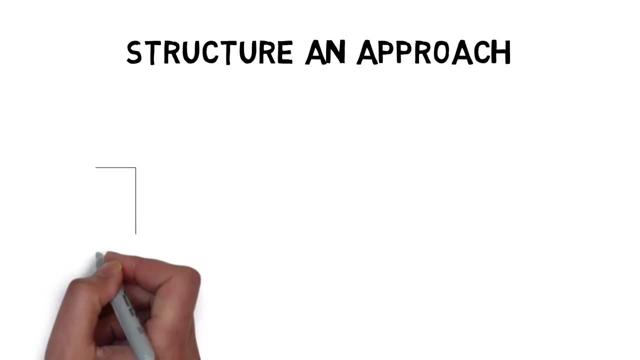 estimation question. Once you have the structure down, you just need to make assumptions and estimates of what numbers to use. That part is easy. The structure is the make or break of the problem and will require some creative brainstorming. There are an infinite number of ways to structure your approach. 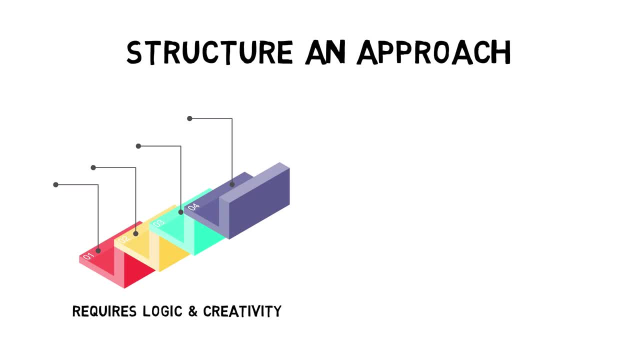 number of ways to structure your approach to the problem and there is no one right answer. Pick whichever approach is easiest for you. As long as your approach gets you to a final answer, your approach should be perfectly fine. Here is one approach we can take. Let's start with the US population and then estimate. 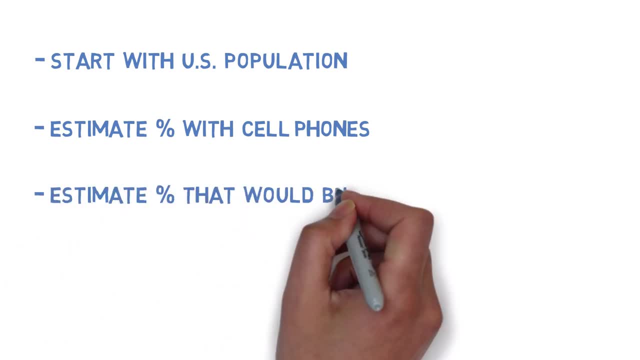 the percentage that have cell phones. Next, we'll estimate the percentage of people with cell phones who would purchase insurance. We'll then estimate how much cell phone insurance costs per year. Finally, we'll multiply all of these figures together to get our market size. 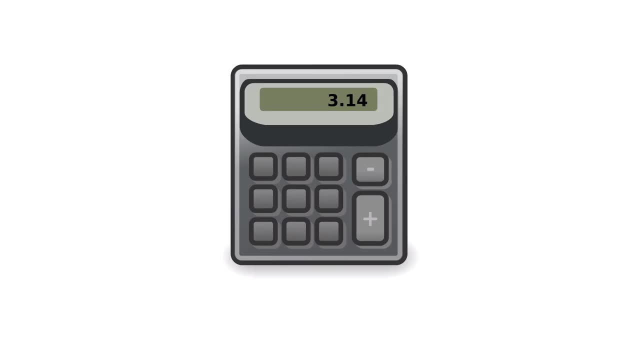 Executing on the math should be fairly straightforward. There is no complex or advanced-level math involved in case interviews. All the math that you need to know is at a middle school level, So make sure you do your calculations correctly, especially paying a. 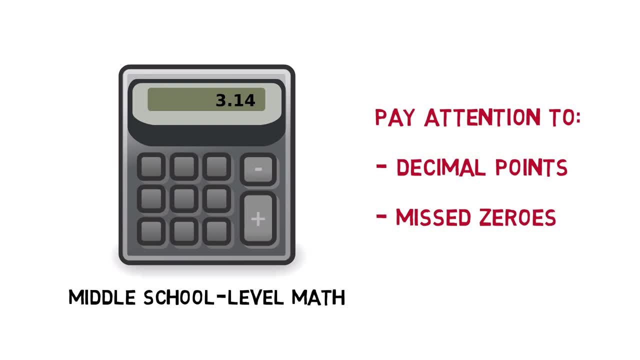 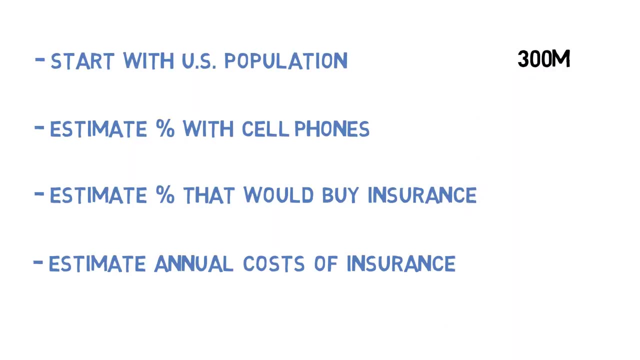 lot of attention to if you have misplaced a decimal point or missed a zero in your calculation. These math mistakes are by far the most common. Let's execute on the calculations for our problem. We'll start by assuming that the US population is 300 million people. This is a figure that most people memorize and 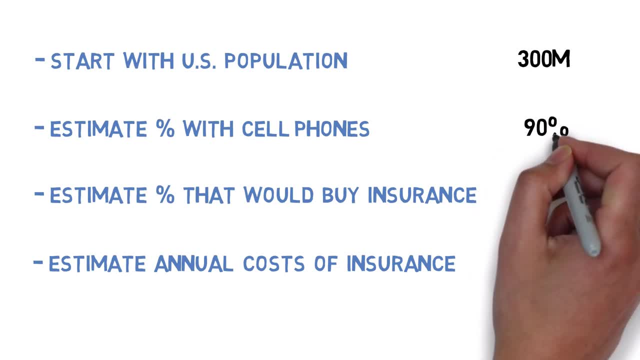 use as a starting point. We estimate that 90% of the US owns a cell phone, so 270 million people own a cell phone. Of those that own a cell phone, perhaps only 30% would buy cell phone insurance. That leaves 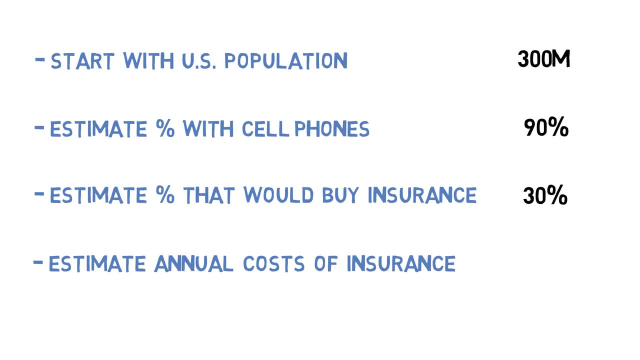 us with 81 million people that would buy cell phone insurance. We might estimate that cell phone insurance costs about $25 a month or $300 a year. So multiplying 81 million customers with $300 gives us a market size of $24.3 billion. 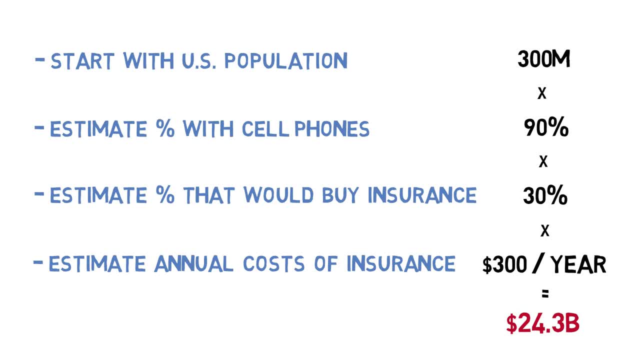 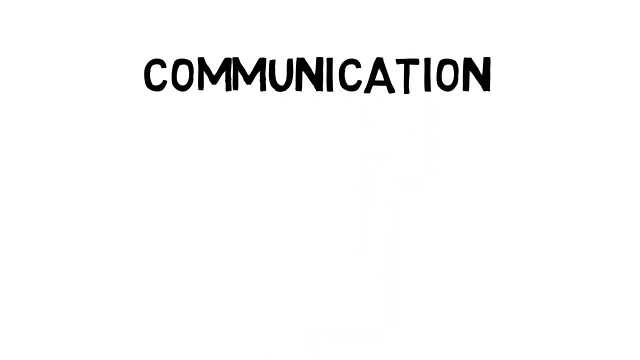 This market sizing problem was not too difficult. Structuring our approach made the execution of the math very simple. Moving on to communication, it is important that you are not making calculations in silence. You should be talking with the interviewer, walking them through which step of the calculation. 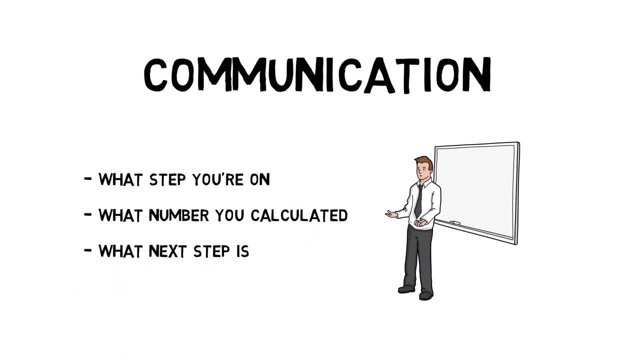 you are doing, what number you ended up calculating and what the next calculation step is. If the interviewer had their eyes closed, they should be able to follow your math and know exactly what you are doing. It may be helpful to re-watch the portion of this video where I walked you through the 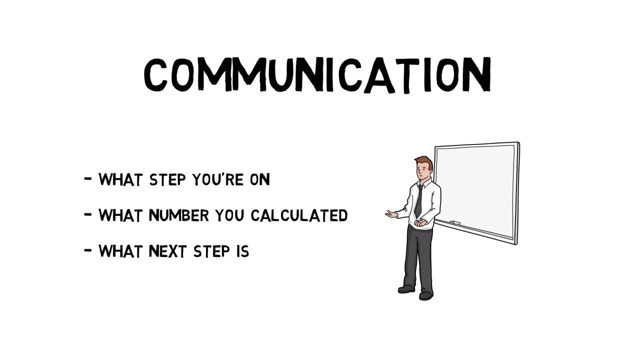 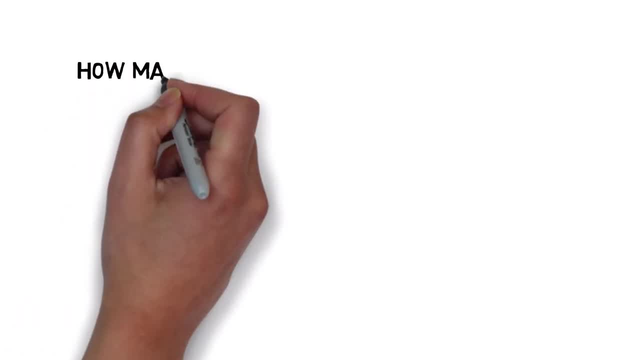 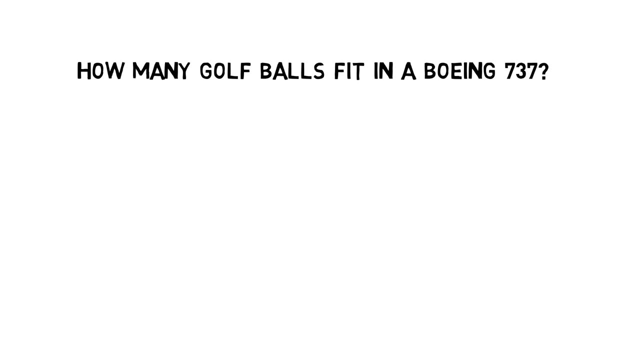 approach and calculations. That is exactly how you should be communicating and presenting to the interviewer. With this problem wrapped up, let's return to our original question: How many golf balls can fit in a Boeing 737?? This one is a bit more tedious to solve. 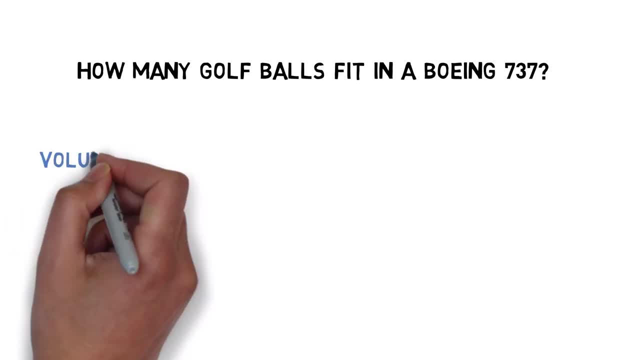 The structure to our approach is actually quite simple. If we know the volume of the airplane and the volume of a golf ball, we can calculate how many golf balls fit in a plane. We can divide these two numbers to figure out our answer. Estimating the volume of a golf ball is simple, but the process to estimate the volume of 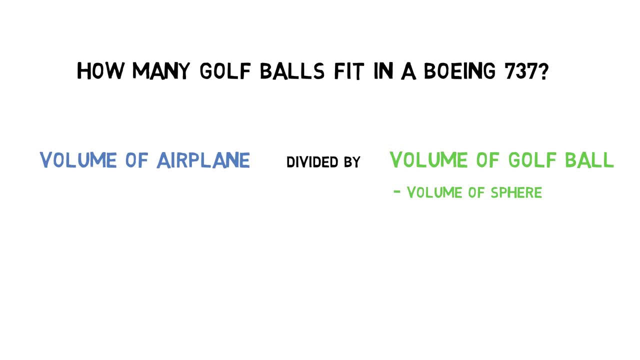 an airplane is more tedious. We might model the airplane as a long rectangular prism estimating the length, height and width. We can then estimate what percentage of that volume is empty, so that we exclude volume that is occupied by seats and other solid.